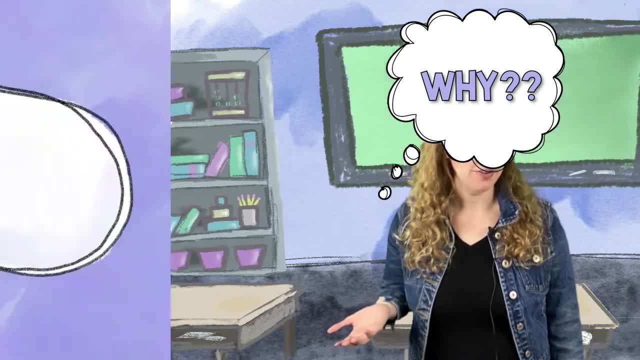 Why is it important we know how to find the perimeter of a rectangle. Perimeter is used in real life in a variety of ways. For example, if you need to build a fence, you need to know that the perimeter of a rectangle is the same as the perimeter of a fence. If you need to build a, 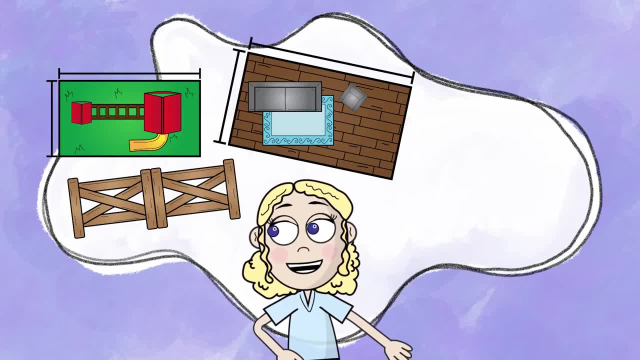 fence, you need to know that the perimeter of a fence is the same as the perimeter of a fence perimeter around a yard. If you need to build a wall or a room, you need to know the perimeter of that room. or even a picture frame, You need to know the perimeter to frame the picture. 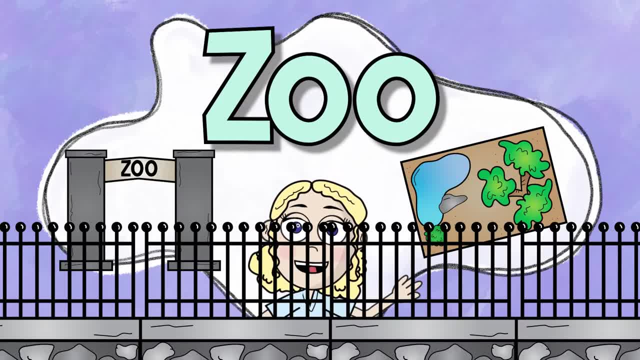 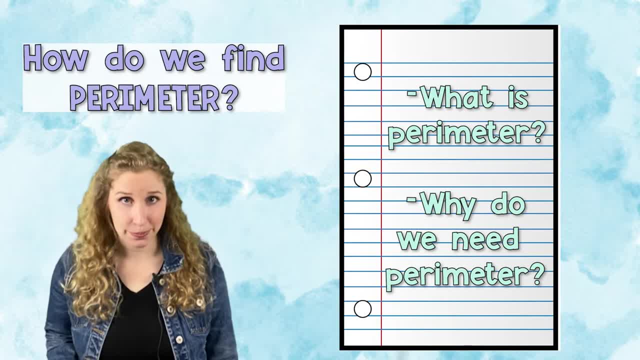 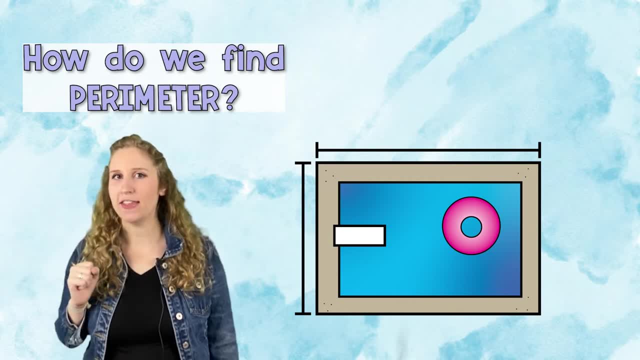 Let's just say we are all thankful that the person at the zoo knew what perimeter is. All right, so now we know what perimeter is and why we need it. How do we find perimeter? I'm going to show you how we find perimeter and I want you to see what I'm doing. Let's try this one. 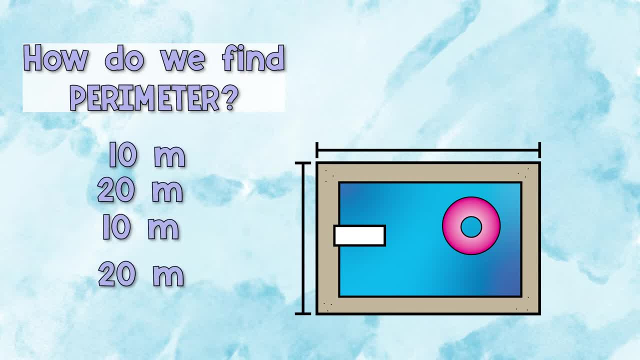 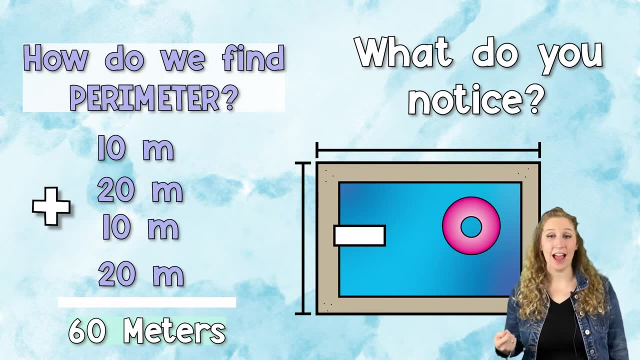 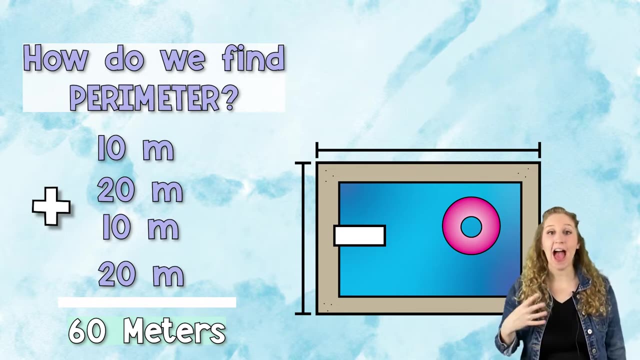 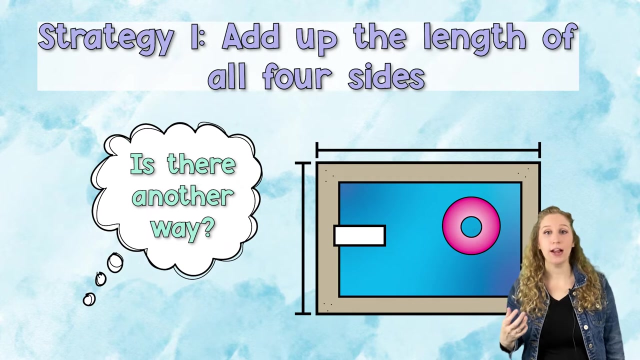 What do you notice? That's right, I'm actually adding all four sides up of this rectangle. So one way you can find perimeter is actually by adding up all four sides. But I want you to stop and think for a second. Is there a way, if we're talking about a rectangle, 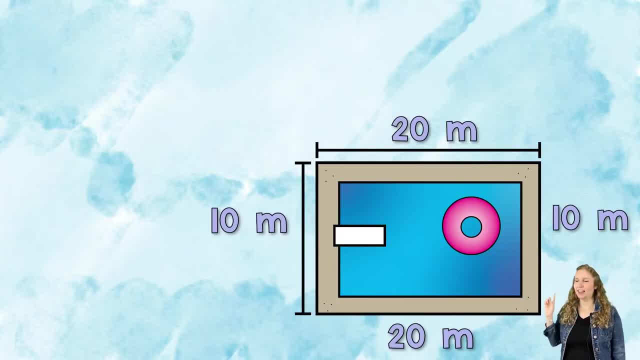 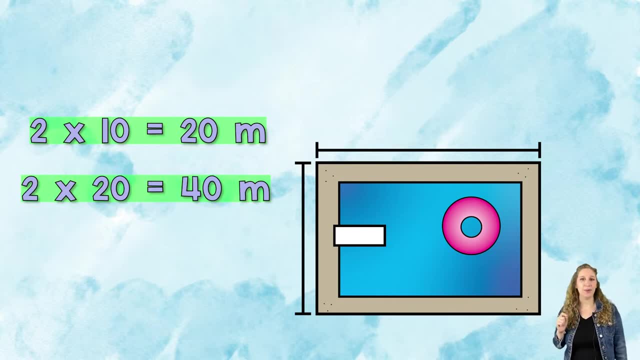 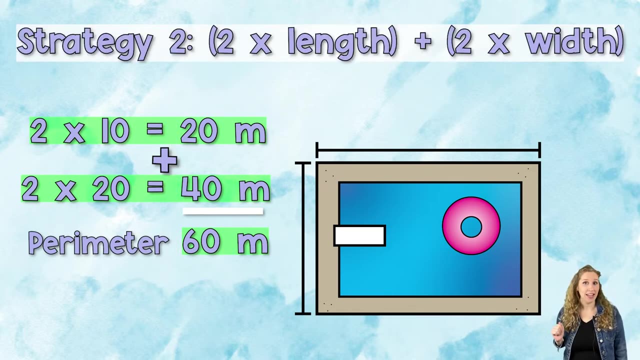 we can find the perimeter. I'm going to show you another way. Let's look at this same rectangle. What am I doing? Ah, As you notice, you can actually write a separate equation to find the perimeter of the rectangle. So you can do 2 times length plus 2 times width. 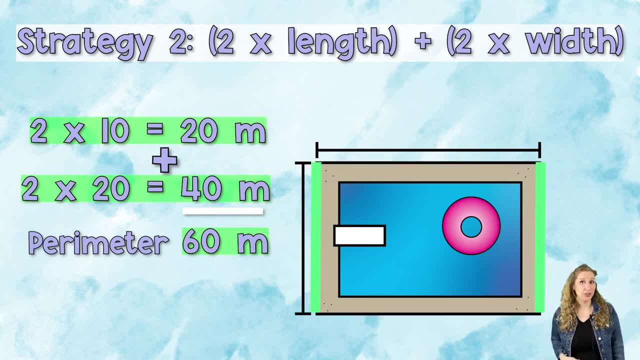 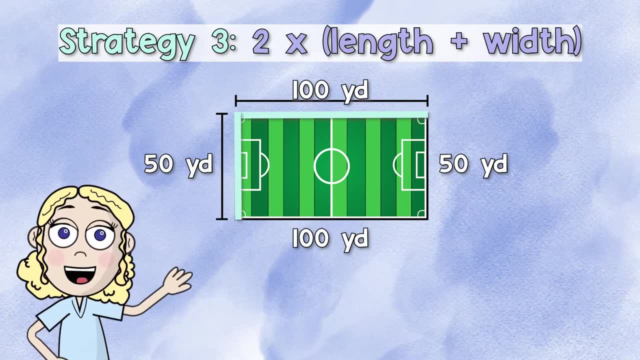 Because, look, There's two lengths and there's two widths. There's actually a third way to find perimeter too. What you can do is you can actually add the length and the width of this rectangle and then multiply it back. There we go. If you're in the circumstances of a big circle, that's okay. 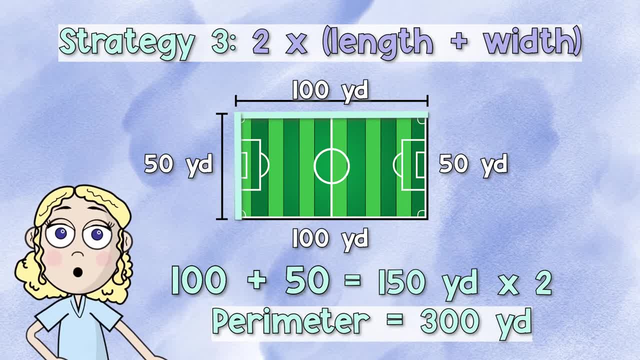 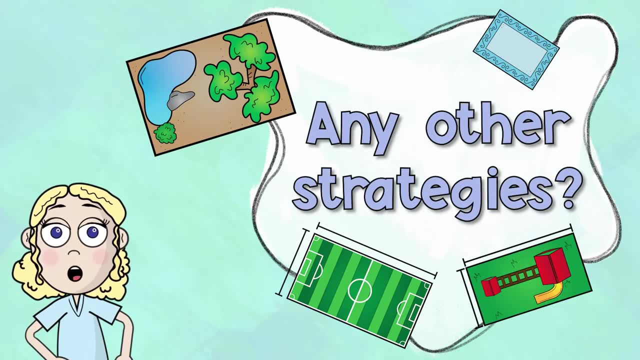 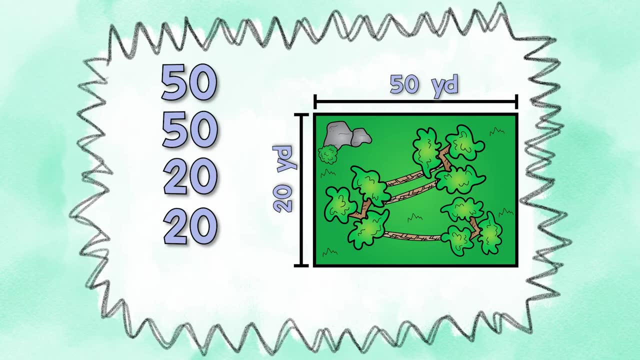 by two Here. watch, That's. the best part about math is you can find a strategy that works best for you. Do you think there are any other strategies to find the perimeter of a rectangle? Let's try a few together. The length of this zoo enclosure is 50 yards. The width is 20.